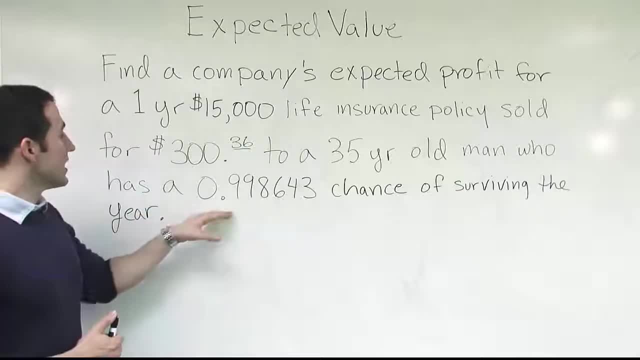 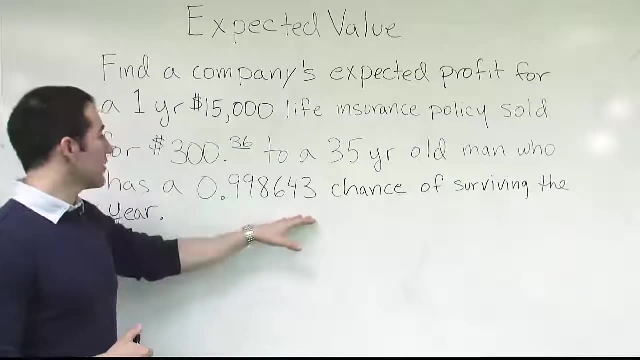 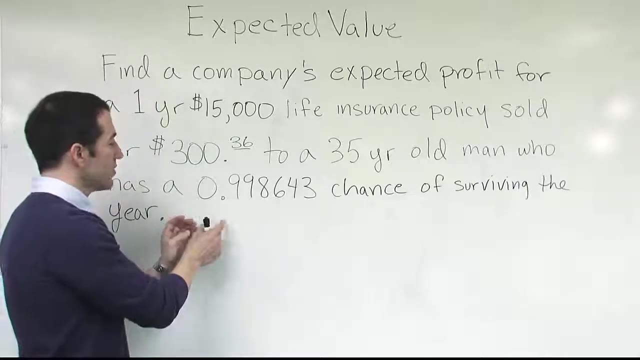 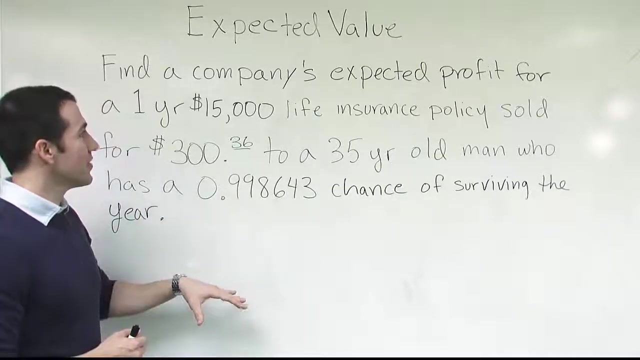 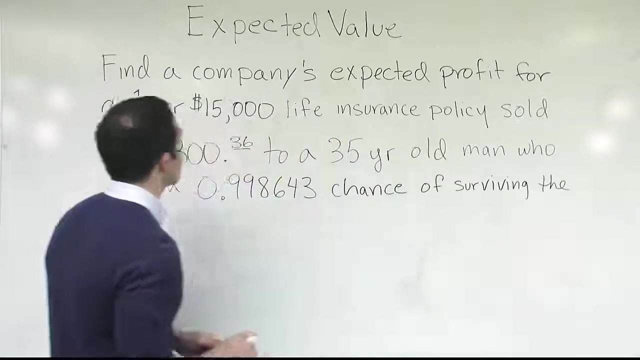 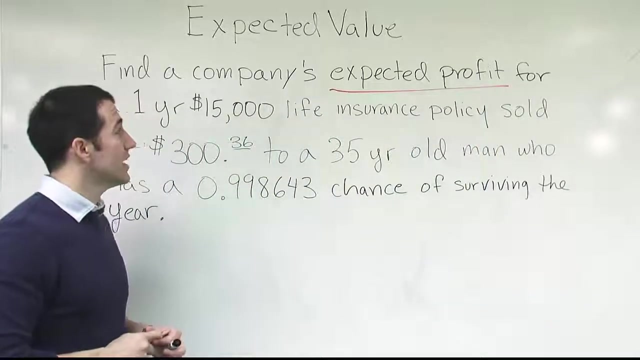 So let's read the problem and see what they're trying to get us to find. It says: find a company's expected profit for a one-year $15,000 life insurance policy sold for $300 and $300.. So let's read the problem and see what they're trying to get us to find. It says: find a company's expected profit for a one-year life insurance policy sold for $300 and $300. 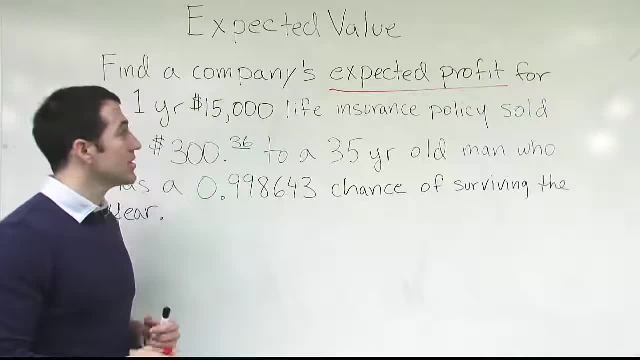 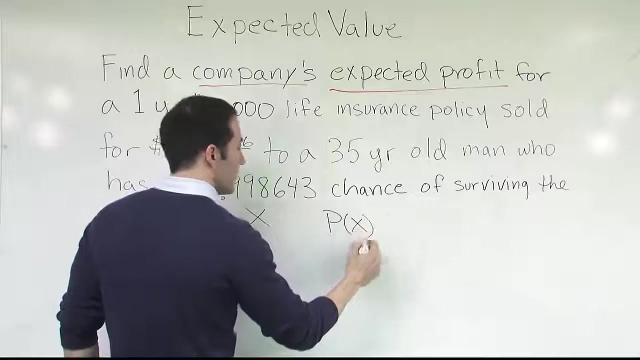 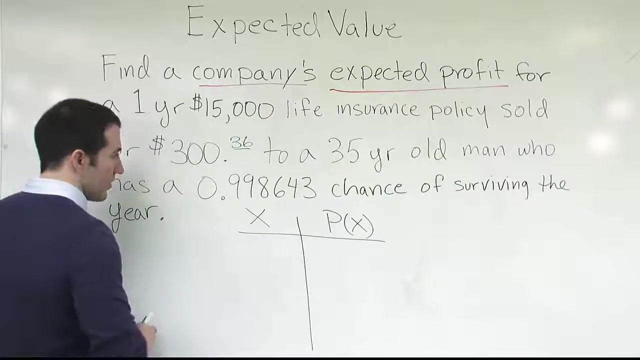 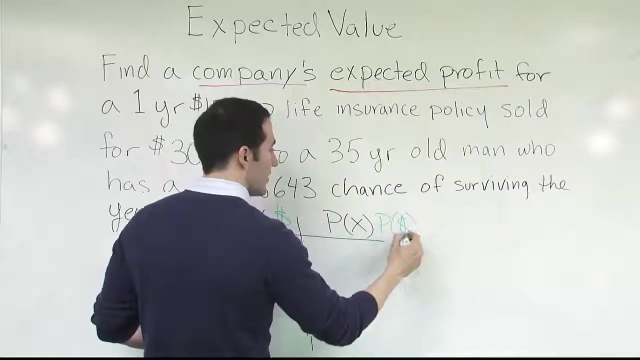 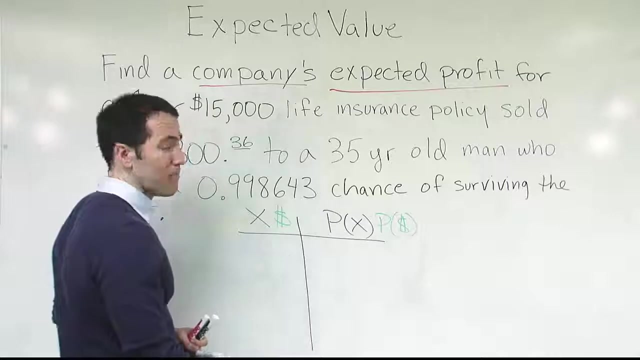 So let's read the problem and see what they're trying to get us to find. It says: find a company's expected profit for a one-year $15,000 life insurance policy sold for $300 and $300.. So let's read the problem and see what they're trying to get us to find. It says: find a company's expected profit for a one-year $15,000 life insurance policy sold for $300 and $300. 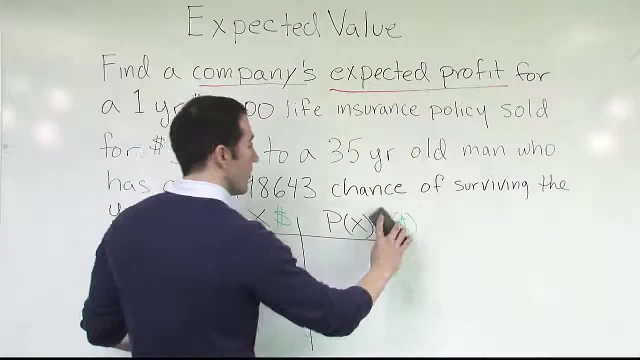 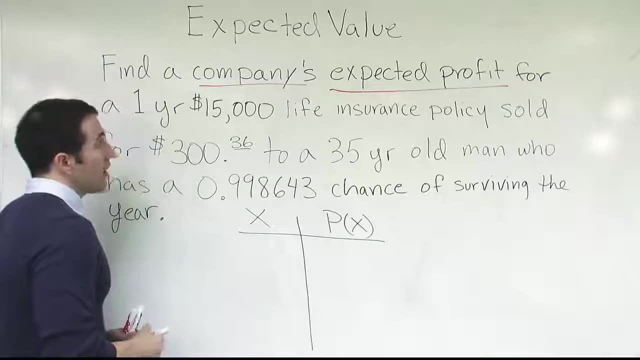 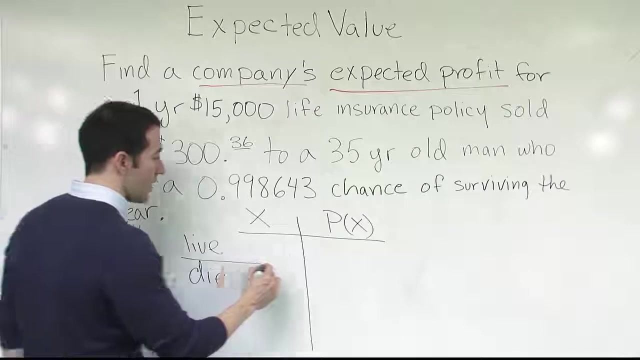 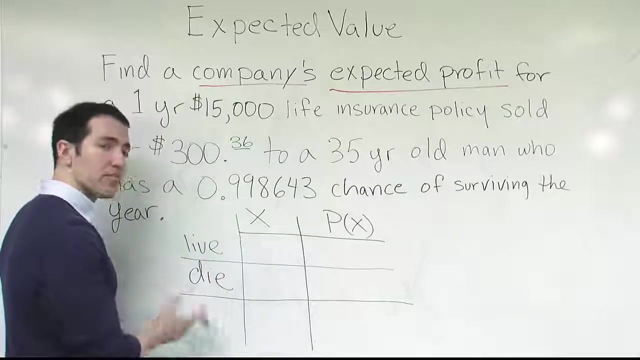 So let's read the problem and see what they're trying to get us to find. It says: find a company's expected profit for a one-year $15,000 life insurance policy sold for $300 and $300.. So let's read the problem and see what they're trying to get us to find. It says: find a company's expected profit for a one-year $15,000 life insurance policy sold for $300 and $300. 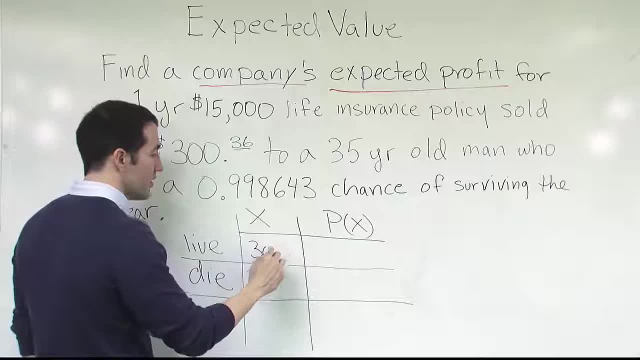 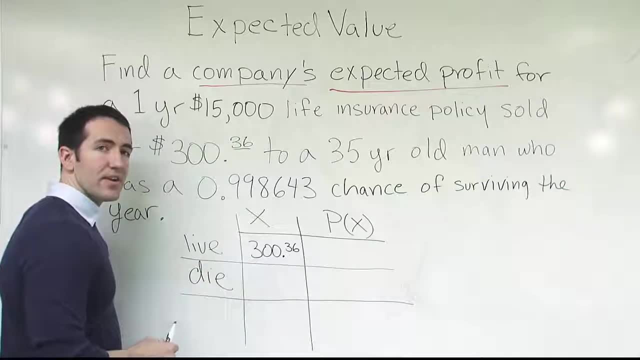 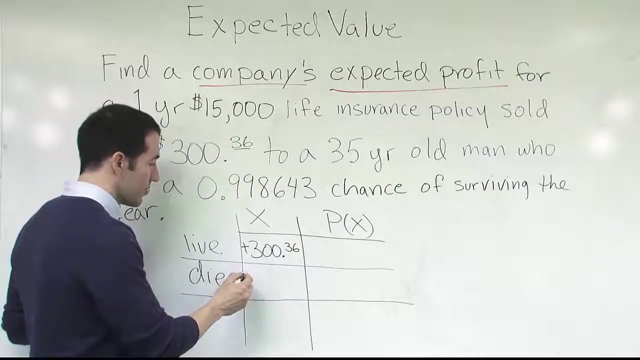 So let's read the problem and see what they're trying to get us to find. It says: find a company's expected profit for a one-year $15,000 life insurance policy sold for $300 and $300.. So let's read the problem and see what they're trying to get us to find. It says: find a company's expected profit for a one-year $15,000 life insurance policy sold for $300 and $300. 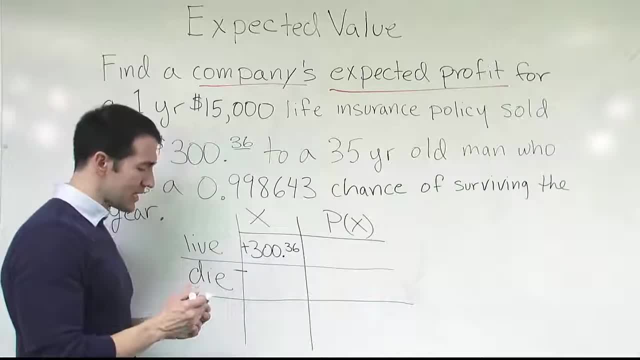 So let's read the problem and see what they're trying to get us to find. It says: find a company's expected profit for a one-year $15,000 life insurance policy sold for $300 and $300.. So let's read the problem and see what they're trying to get us to find. It says: find a company's expected profit for a one-year $15,000 life insurance policy sold for $300 and $300. 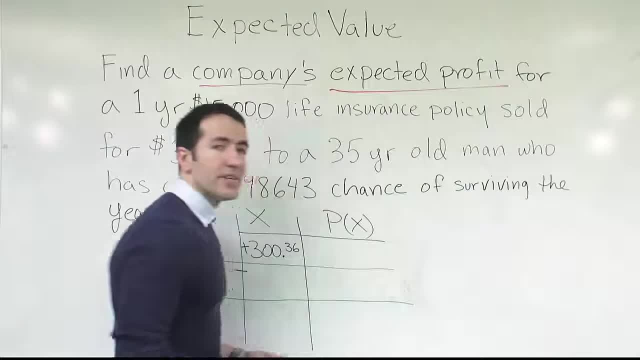 So let's read the problem and see what they're trying to get us to find. It says: find a company's expected profit for a one-year $15,000 life insurance policy sold for $300 and $300.. So let's read the problem and see what they're trying to get us to find. It says: find a company's expected profit for a one-year $15,000 life insurance policy sold for $300 and $300. 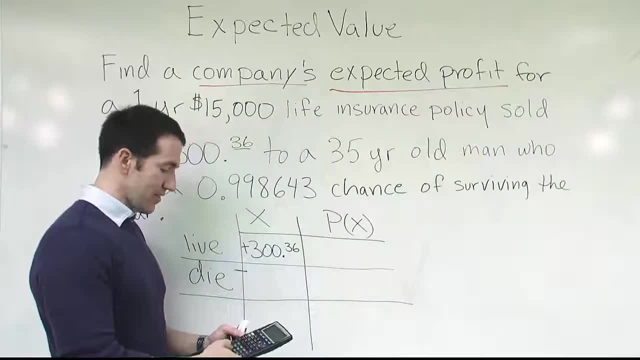 Of course, what you want to do is you want to take your $15,000 and you want to subtract off your $300.36 from that number, give you your $14,699.64.. You have to do that because the company is not going to fork back over the $300. the person 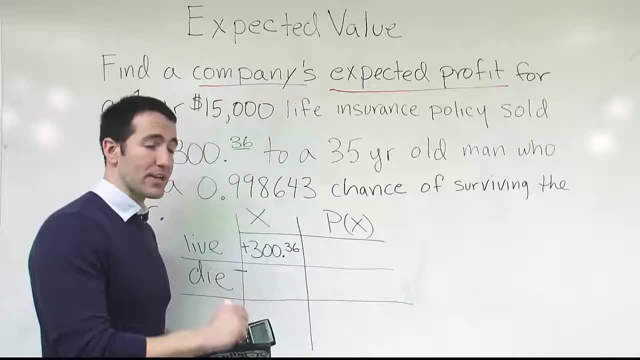 paid for the policy. You're going to keep that sort of in the back pocket. You're going to write a check for $15,000, so even though they're paying $15,000, they still got that $300 in their back pocket. 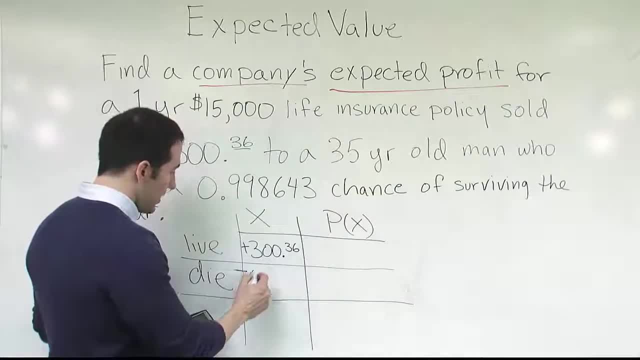 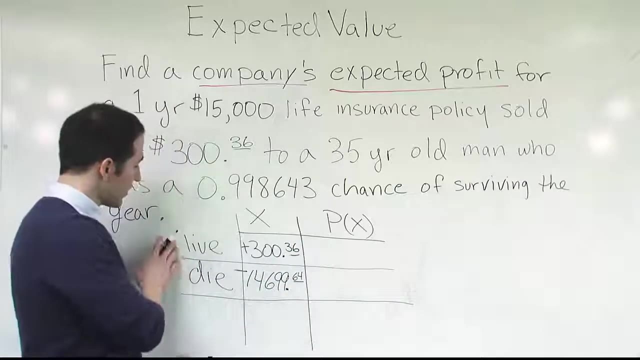 Let's put that number in then on the table, The proper number again is $14,699.64.. We now have the proper dollar amounts listed in the table. Now, from here we're going to plug in the probabilities. Look back at these controlling events over here. live and die. 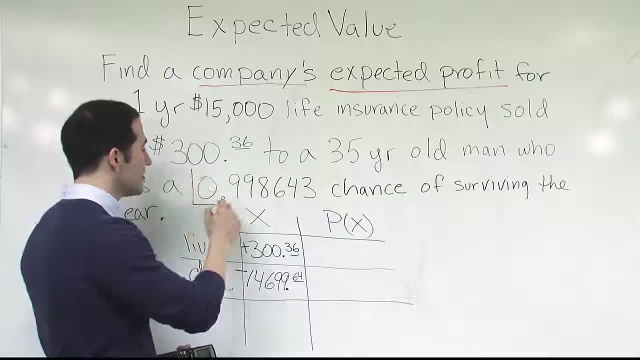 What's the probability? the person lives for the entire year. That always has to be given to you. You can't be expected to know that. That's what the actuaries are for. They'll figure that out for you. We go from the problem. 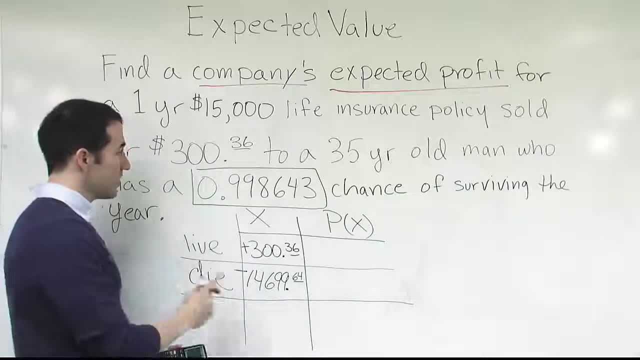 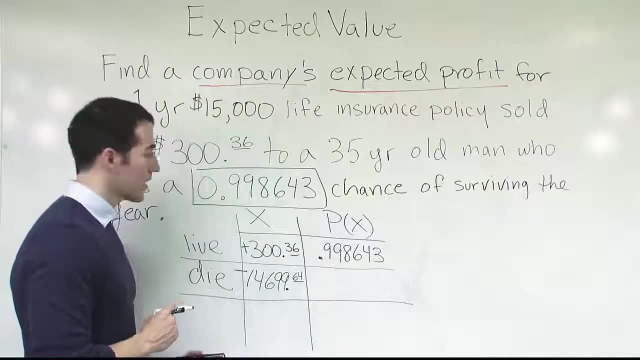 We find this probability, That's, the person's probability of surviving the year, I'm going to go ahead and put in the .998643 into the table. Once I've done that, then I have to figure out what's the chance the person dies. 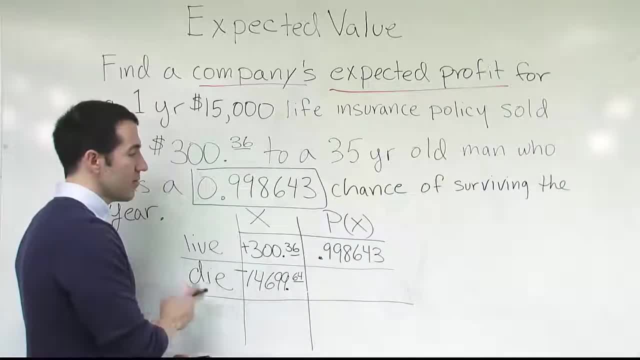 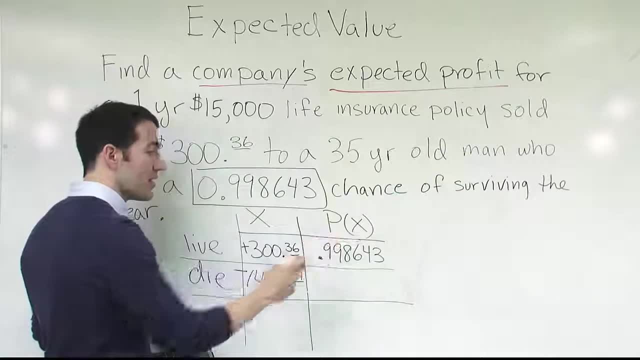 It's an either-or thing: Either you live or you die by the end of the year. It must be that this probability plus this must add up to 100% or 1.. If I take the number 1 and I subtract off that probability, I will end up with the probability. 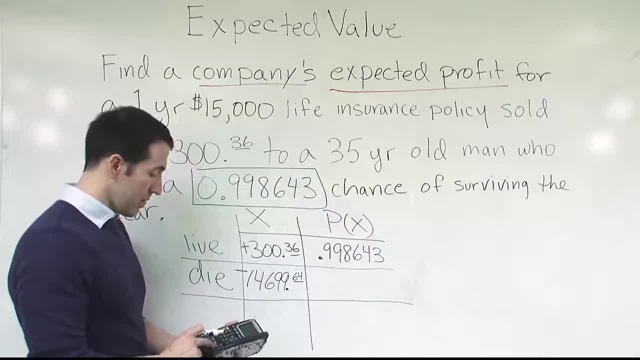 that I die before the end of the year, I have to do 1-.998643.. When I'm done, I get this result: .001357.. That's the probability that the person dies, The probability that they live, the probability that they die. 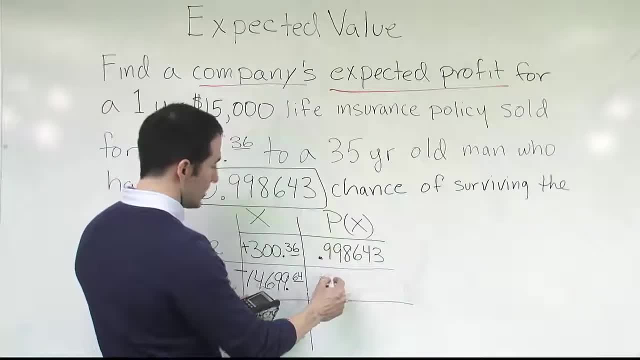 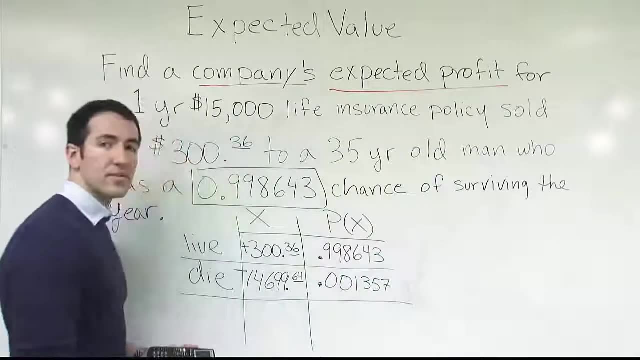 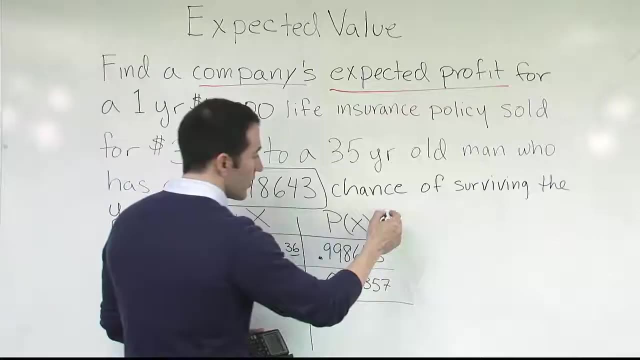 Once you have the table set up- which is probably the hardest part- the rest is just the mechanical calculations From there. that's kind of routine. What you have to do to form the average is to do .998643.. That's the probability that the person dies. 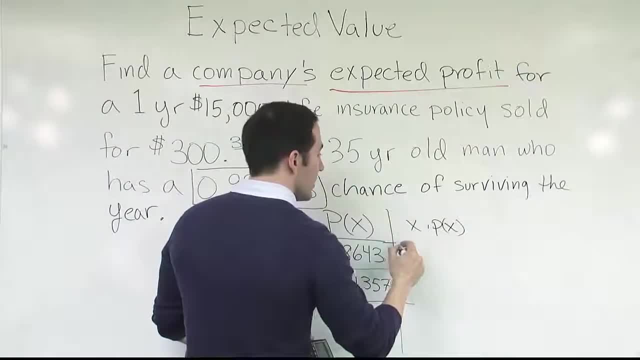 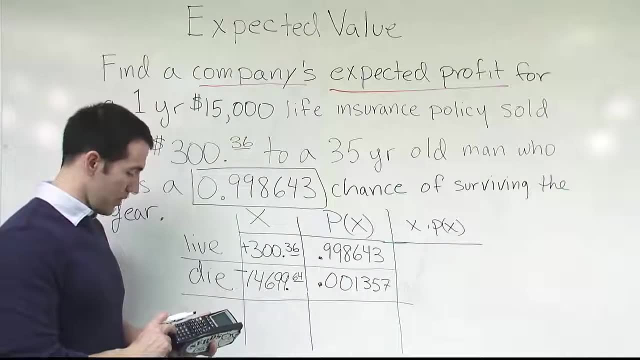 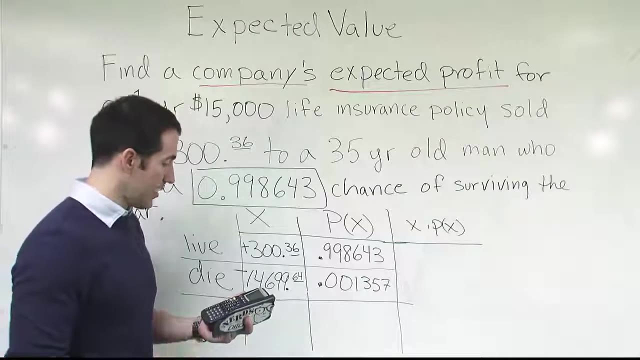 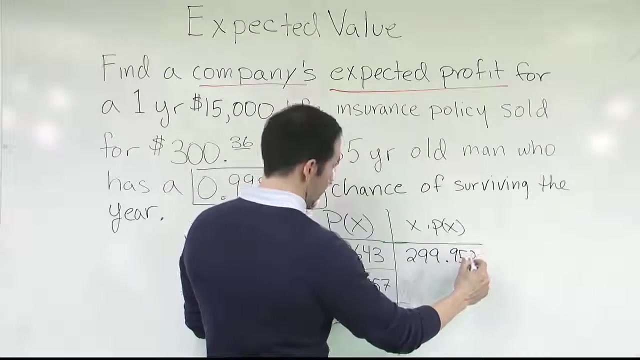 You multiply straight across the x values times the probability values. Let's go ahead and do that. It will be 300.36 times .998643.. When you do that, you get $299.9524115.. About $0.95.. 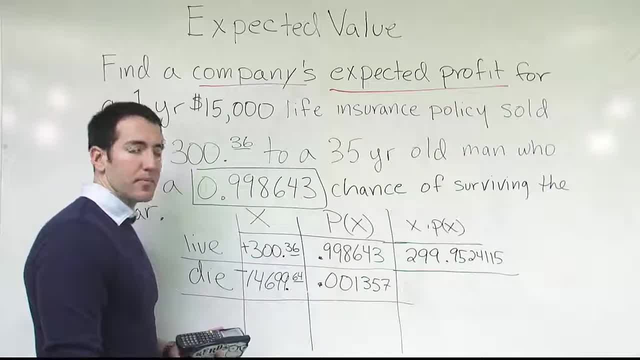 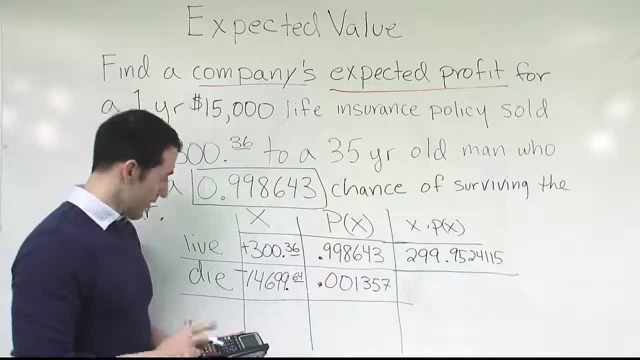 I'm leaving all the decimal places on because we will round off at the end of the problem, not before that. Then let's multiply these two numbers together to get the next column or next row filled in. We have .001357.. 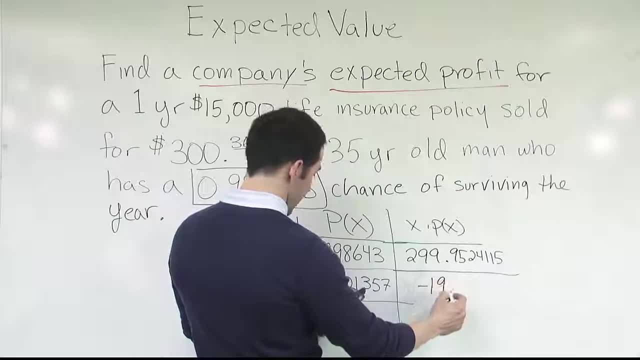 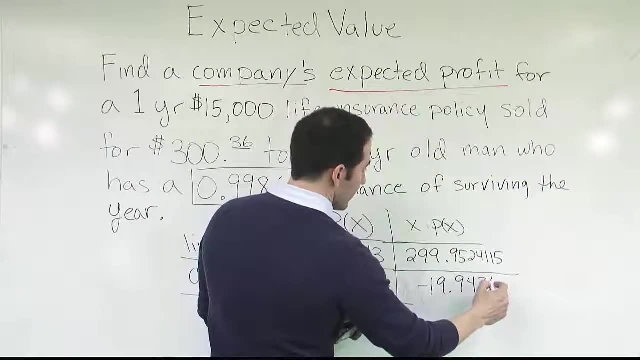 When you're done with that, you get minus $19.95.. It's actually .00947.. That's the probability that the person dies. That's the probability that the person dies. The number is $7141148.. Again, carrying all the decimal places over. 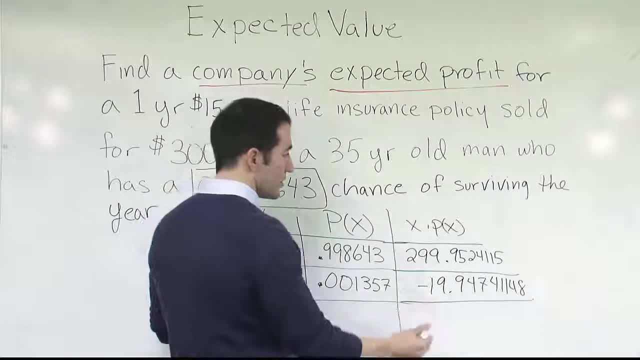 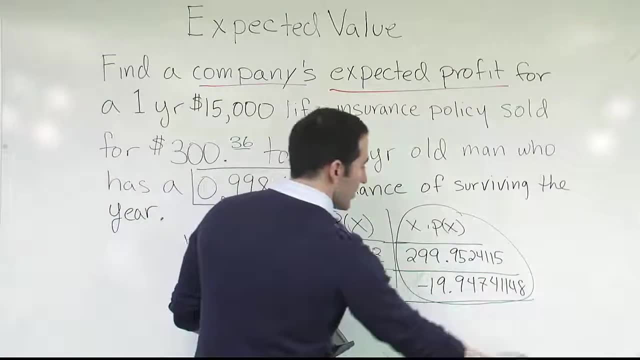 Then, finally, from there to finish the average, we're just going to sum or total this column. To sum that up, we get the average value. The average value is going to end up down here. That's going to be our result.